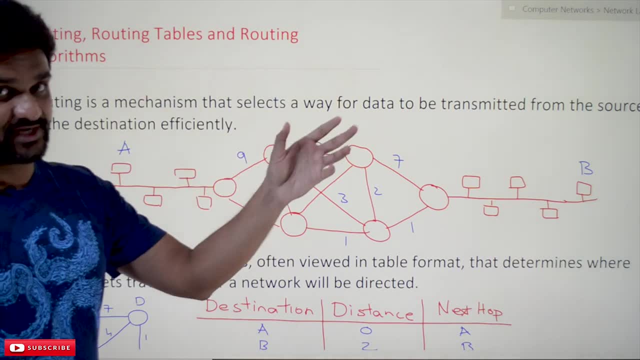 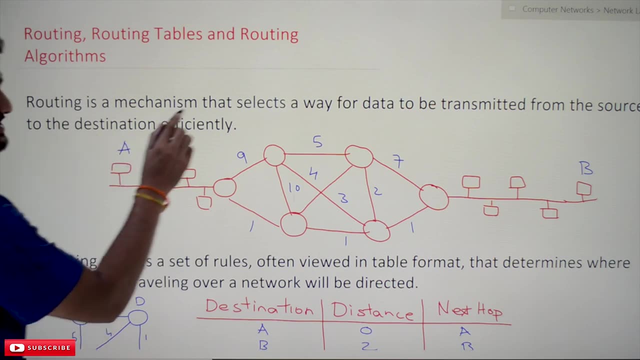 we'll try to understand some of the basic concepts which we need to understand. Okay, so the concept is first, we're going to start with routing. What is meant by routing? Routing is a mechanism that selects a way for data to be transmitted from source to. 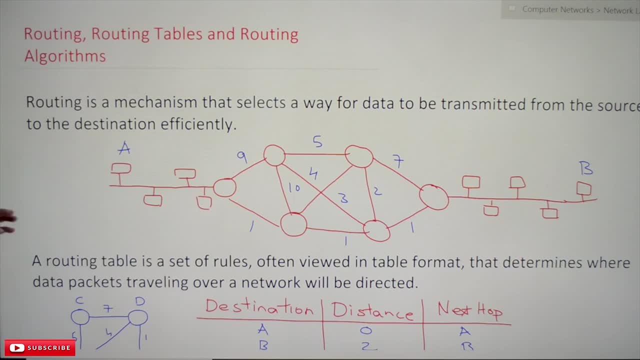 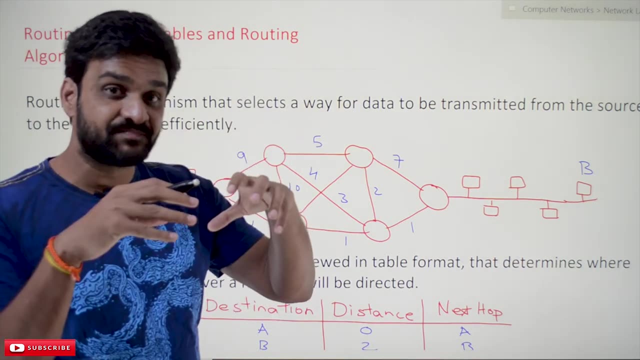 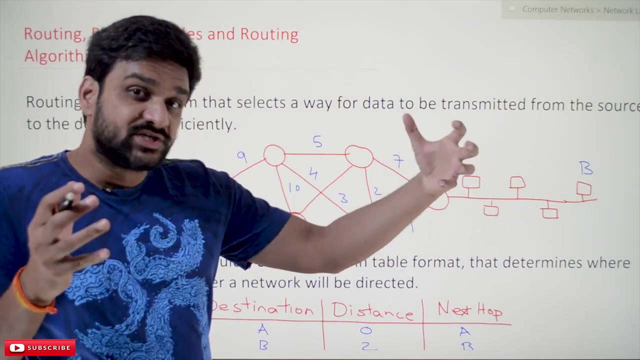 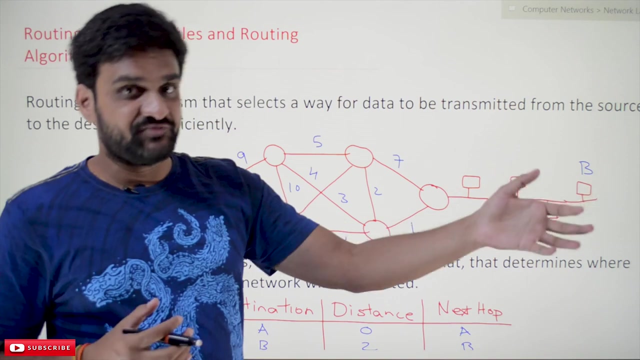 destination efficiently, For example. so so the definition states that routing is a process. routing is a mechanism by which we are going to select a path between the source and destination. among several paths, we are going to select a specific path. that selection of the path is done efficiently, which means 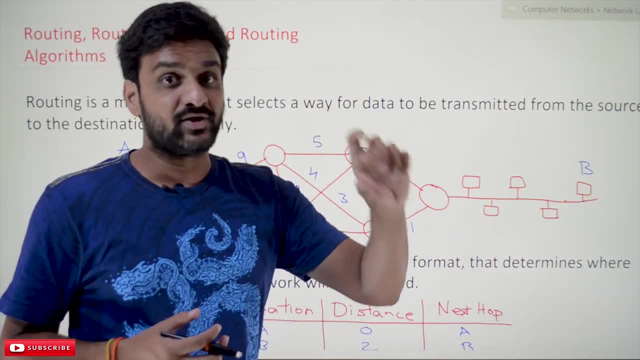 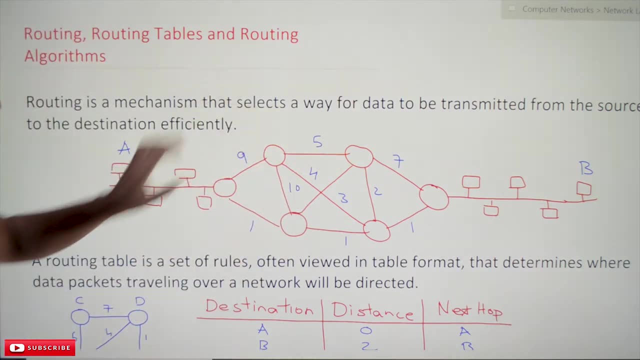 the shortest distance is getting identified. okay, that is what that process of selecting that path is, what we call it as routing. let's try to understand this by using this example. so here we are having a simple network source: a wants to communicate, this is a, this is a system and this system wants to. 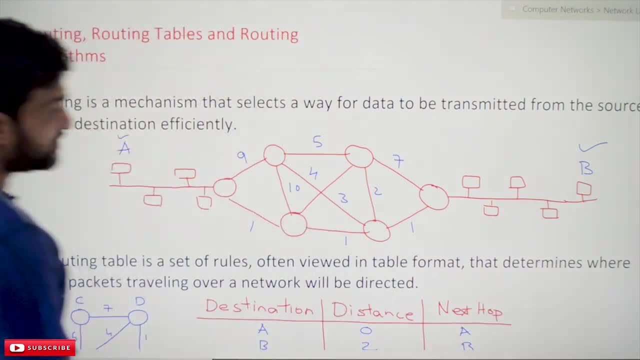 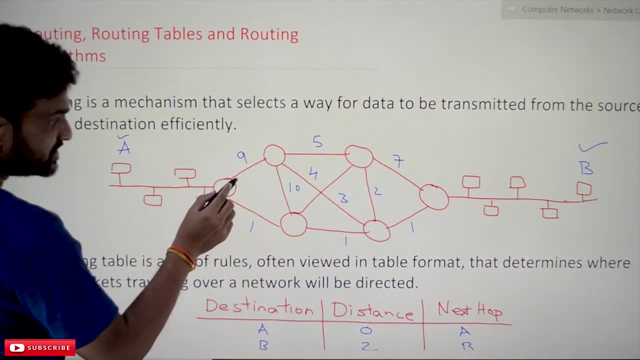 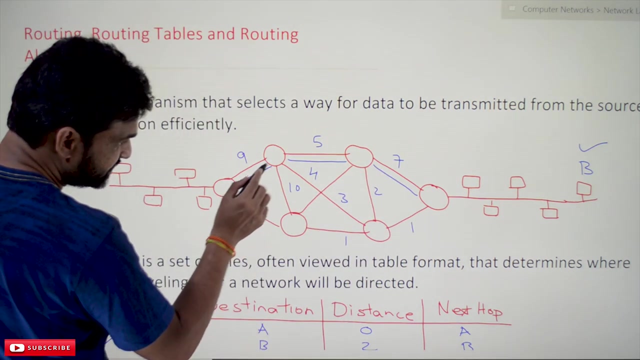 communicate with destination B. now, in order to transmit from A to B, we are having several paths. so what are those paths? so the packet may get transmitted from here to here, here to here or here to here, or it can be transmitted from here to here and after that, here. this way, this way, and 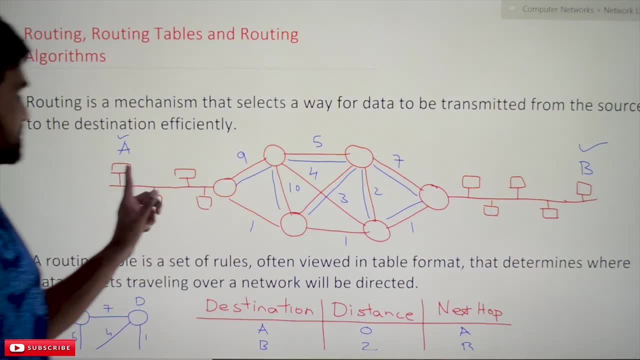 this way, there are different possibilities for this packet to get transmitted from A to B, but among all the things that we have seen in this, cassettes are more hut. those codes are not okay at all. so now which to do when the packet gets transmitted from A to B. askelore 1999. this is a. 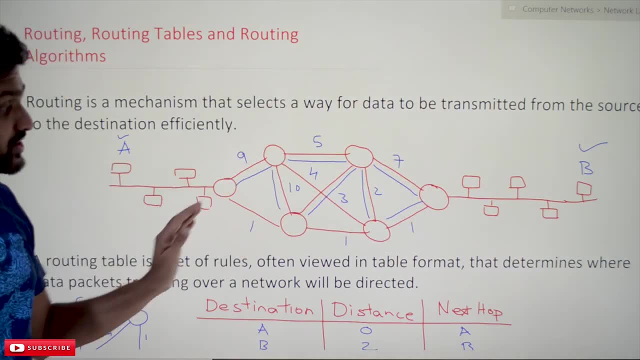 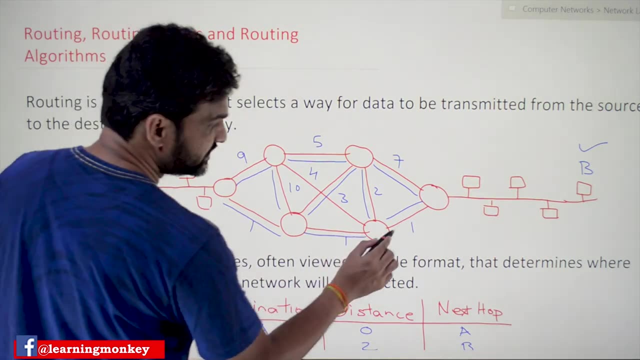 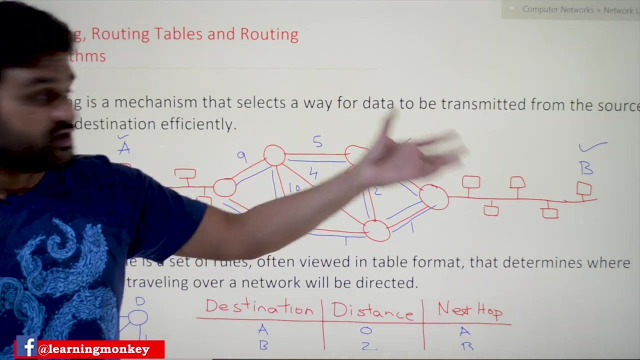 this several paths, it is going to take only shortest path. by just seeing this, we can decide that the shortest path is from here to here, here to here and here to here. so, for example, if you assume that these as the, so these numbers can be assumed in different ways. one of the ways distance. another way is cost. 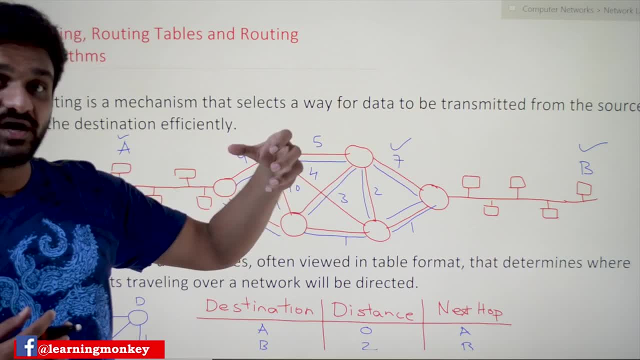 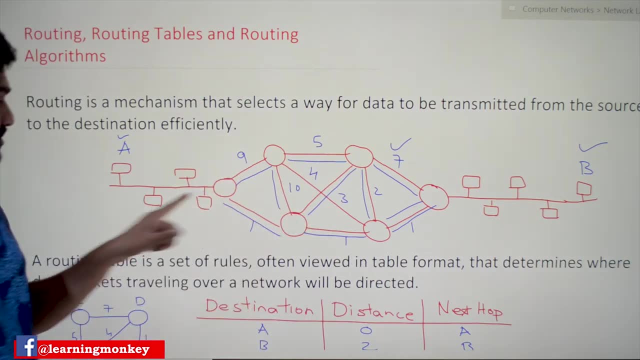 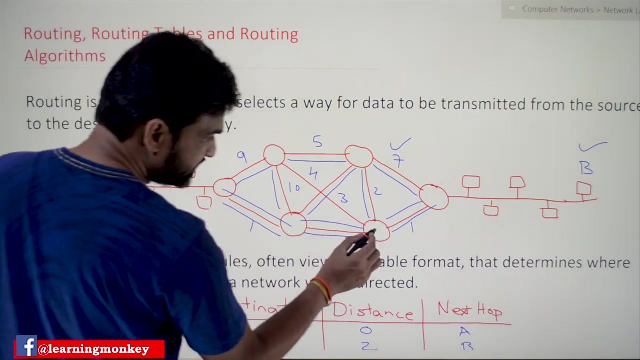 another way is the amount of time. time can also be taken, so there it can be of any type. we are going to consider it as distance, so in order to transmit from A to B, the shortest path is from here to here and after that from here to here. 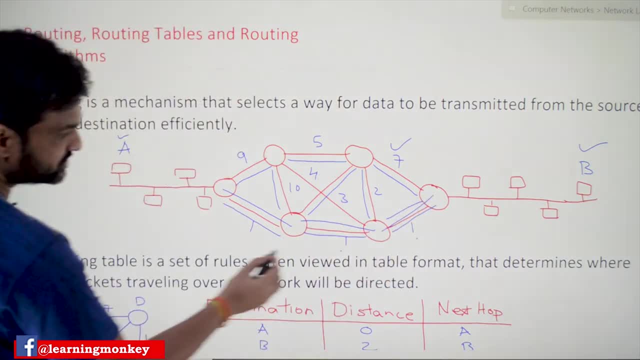 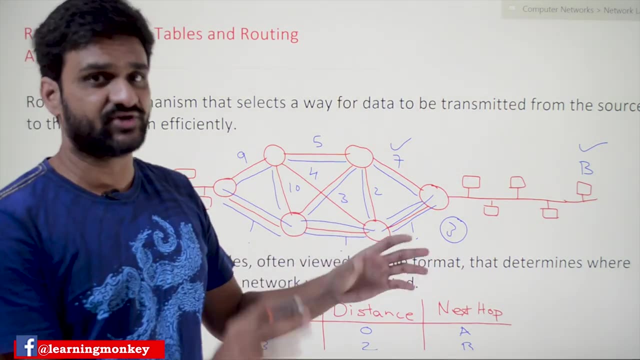 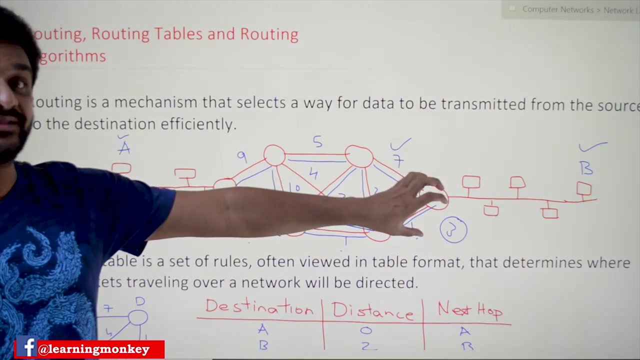 and after that from here to here. so it is going to take a total distance of three units of three units. that unit distance may be a kilometers meters, whatever it may be, so it is going to take an amount of 33 distance. so this is the shortest path efficiently. 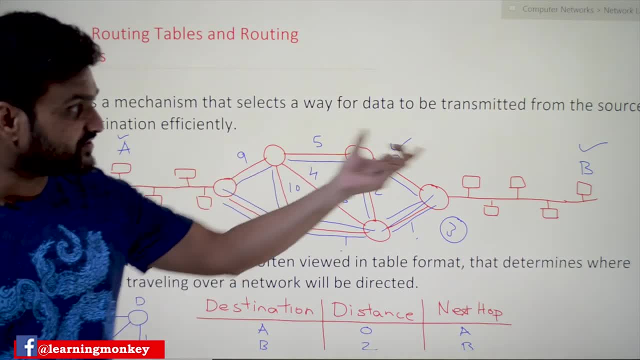 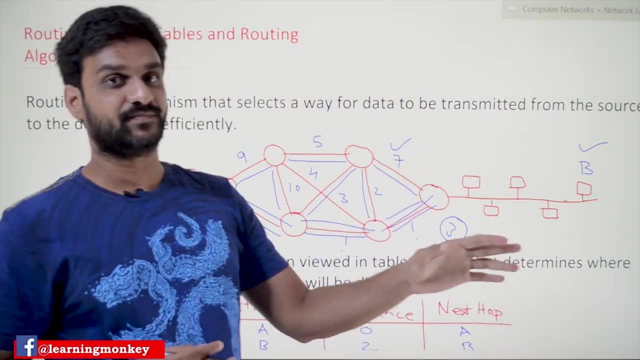 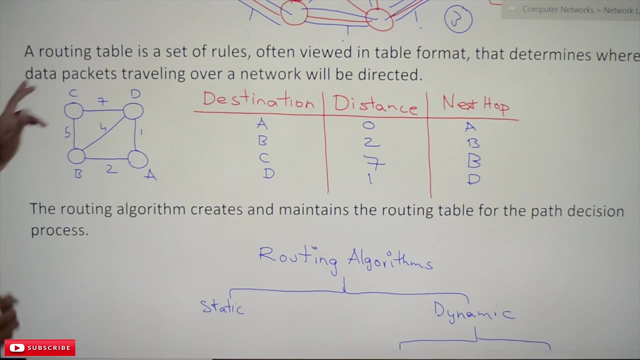 so in order for the data to get transmitted from here to here. 3 is the efficient path, so that process of identifying that path is what we call it as routing. the next definition is a routing table. so what is this routing table? routing table is the set of rules often viewed in the table format, so the 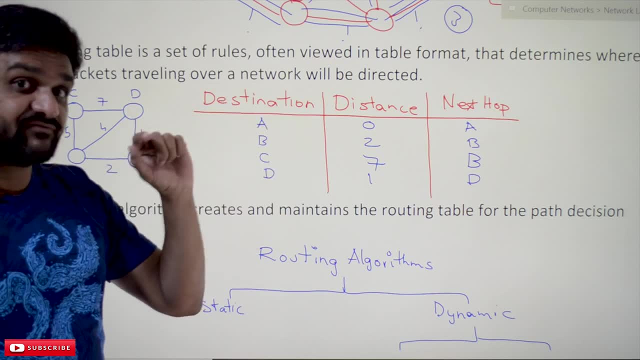 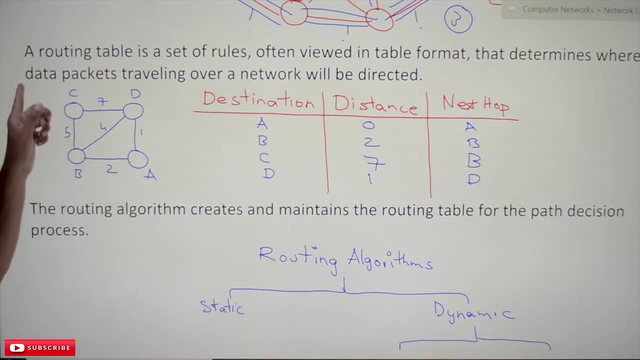 routing table is always in the table format which is having within that it is going to have some set of rules that determines. so what the table determines is where data packets traveling, where the data packets are to be traveled over the network, the data packets that are being traveled over the network will be. 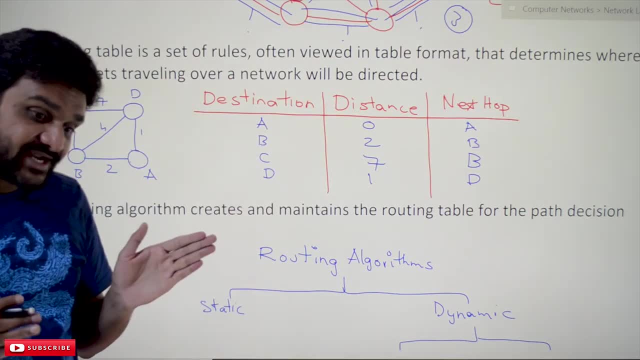 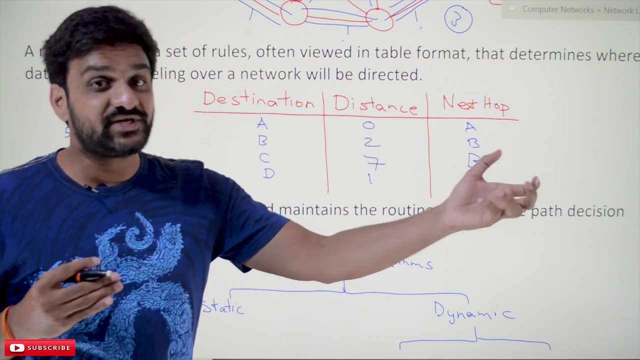 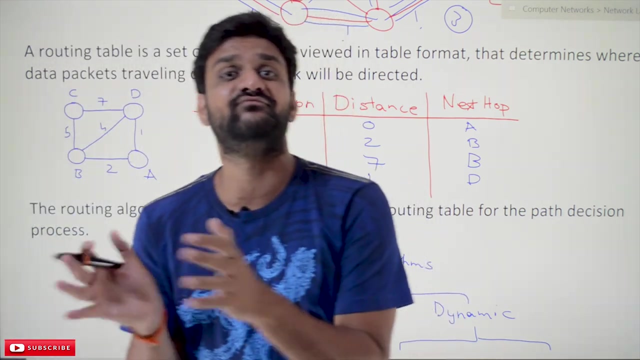 directed. so, using the table, we can direct the data packet that is being transmitted into the network so where the packet has to be transmitted is designed and gets transmitted. that packet is set to the network, so the data by using routing table, and these routing tables will be there on each and every router, so on each. 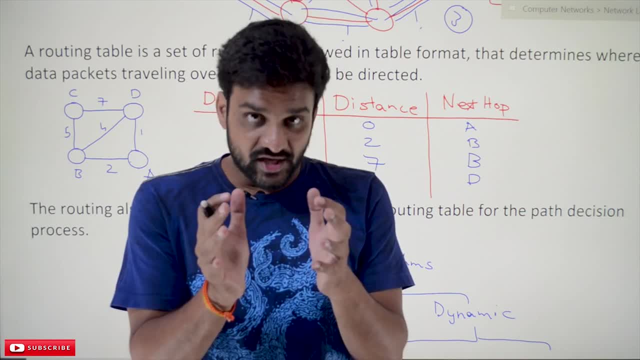 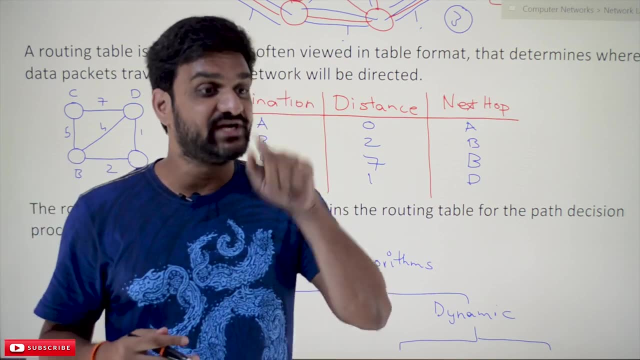 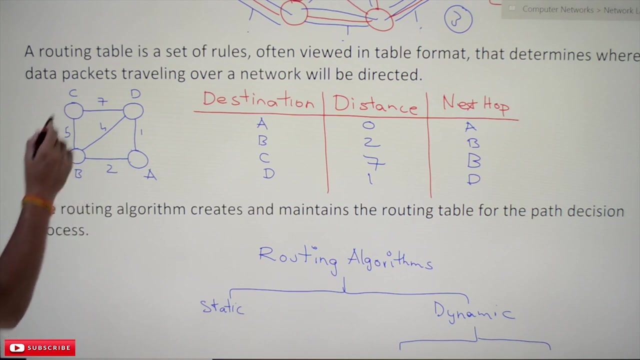 and every router, there will be a routing table. by using that routing table, by using that routing table, the, the packet that is being transmitted will decide where it has to be transmitted. let's try to understand this by using this simple example. here is a network, we are having a. 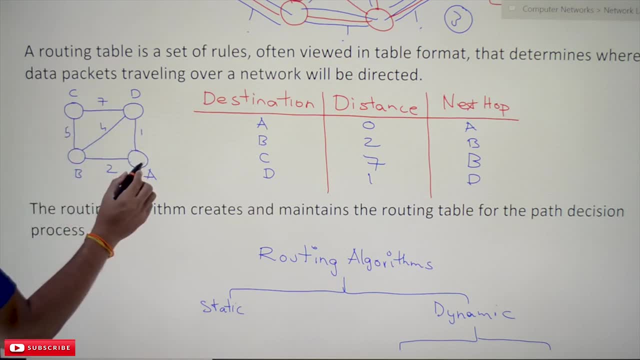 sample network with four nodes and, for example, if the communication, if you want to transmit the data from A to C, A to C, so now the packet is at here, how that packet, so the- let's try to understand this with example here: a wants to transmit the data to C. so what are the best? 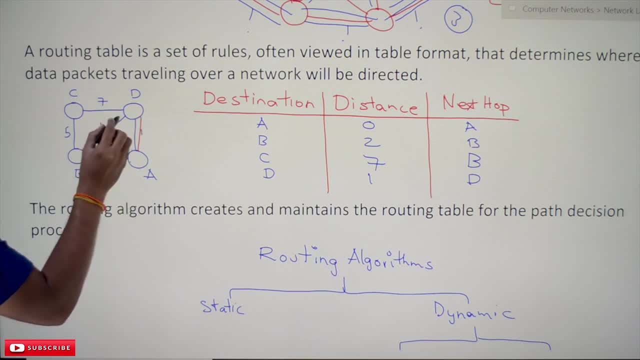 paths that is available. it is from a to B and from D to B, and this is one of the path, not best path, and the other path is a to b and from d to c, and the other path is a to b and b to c. so what is the distance for the first path, from a to d, d to b? 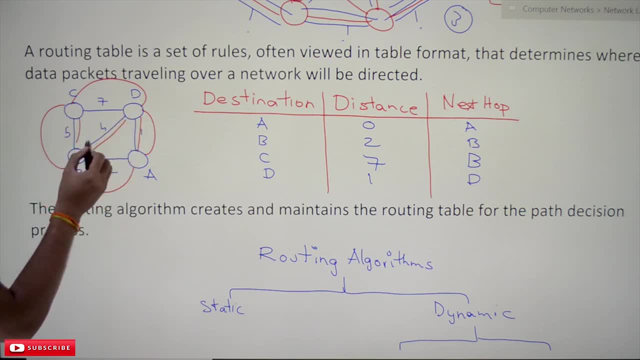 b to c. it is 1 plus 4, 5, 5 plus 5, 10. one of the path is taking 10 distance and a to d and d to d to c. it is 1, 1 plus 7, 8. the other distance is 8 and the other one is a to b and b to c. a to b is: 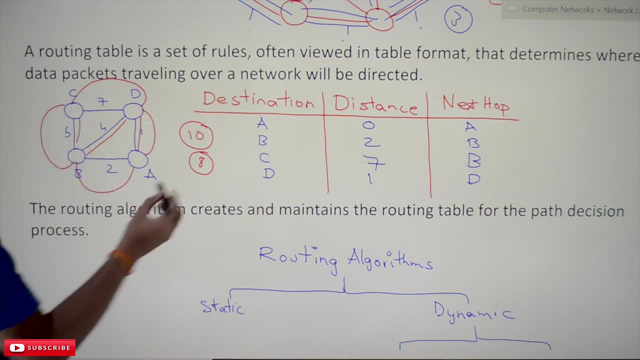 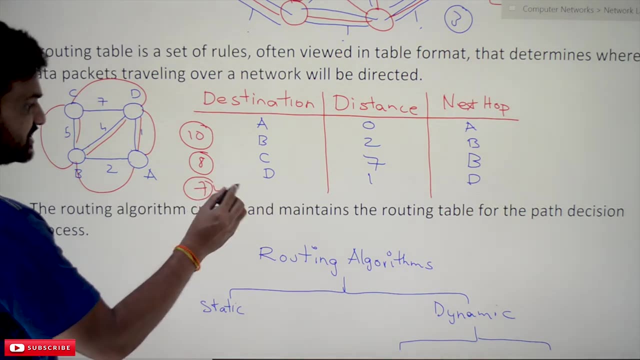 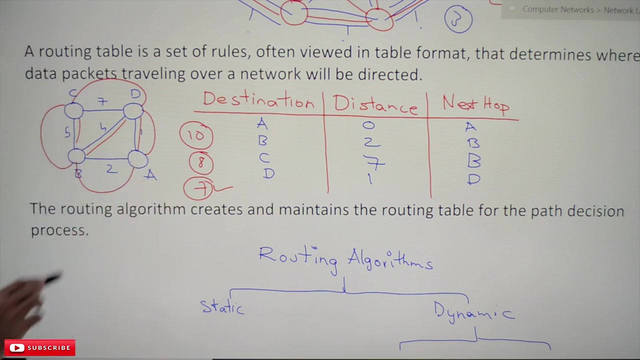 2- from b to c. it is 5. so the total distance is 7. so what is the shortest path among all these? 3- it is 7. so in order for the packet to get transmitted from a to c, what is the next next router to which the packet has to be transmitted? so the possibilities for the packet to get. 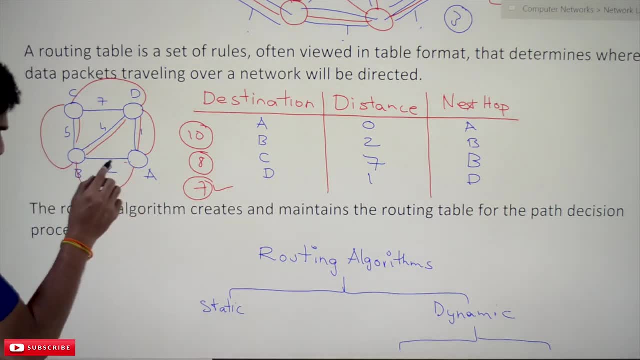 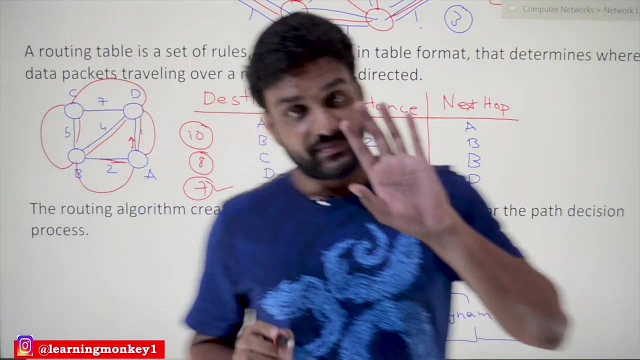 transmitted is. two possibilities are there, so: either to this line or to this line, but but the a will transmit all the packets to c. all the packets to c only through this line. the point that you have to understand is for the packet to get transmitted from a, it is having two options. 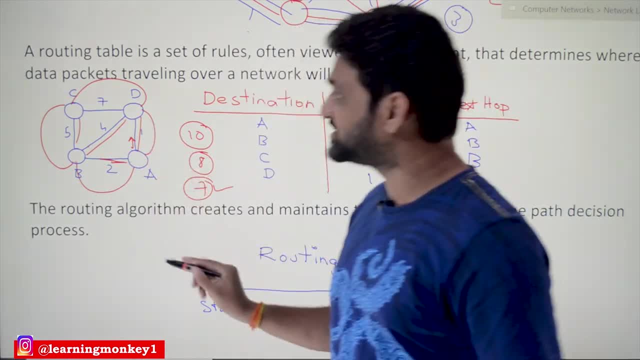 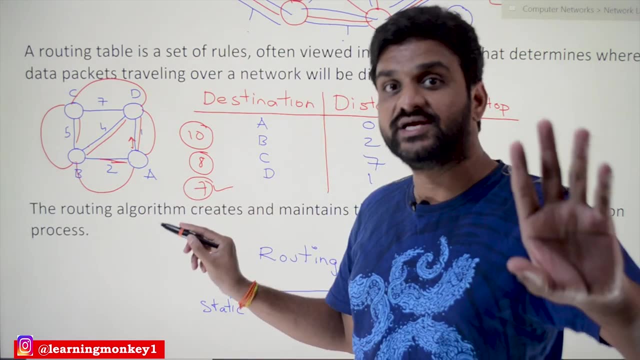 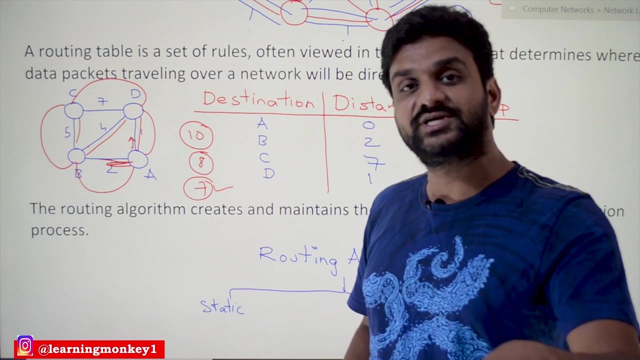 two wire connections are there, one is in this way and the other one is in this way and the other one is this way. but but the packet will. if you want to transmit the packet from a to c, it will always get transmitted through this line. through this line, because if the packet is transmitted. 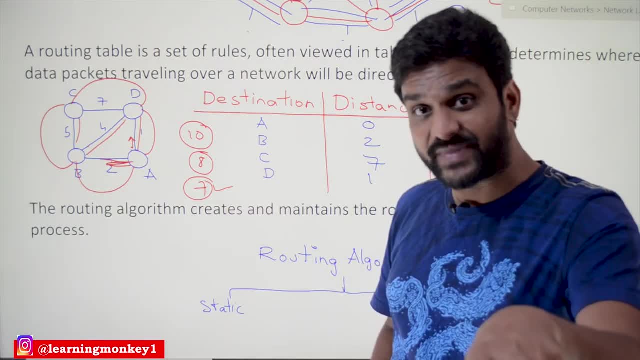 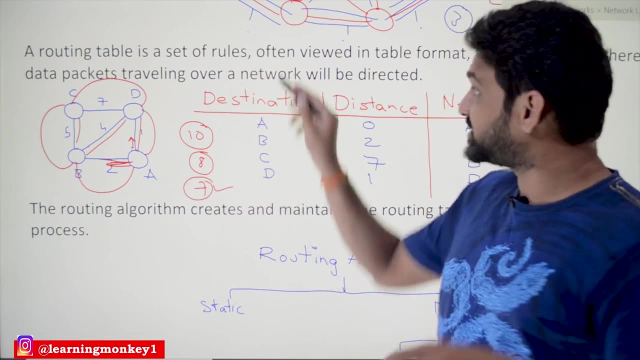 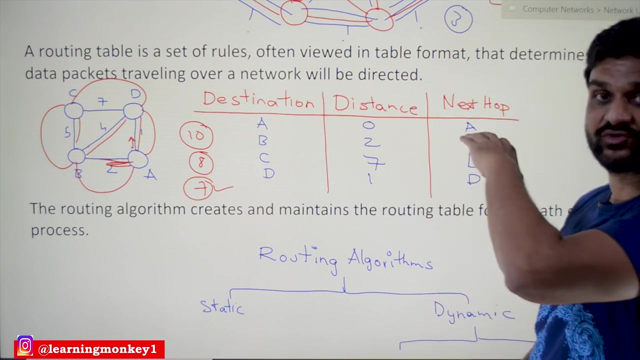 through that line. it is going to get the shortest path. that decision that decisions here. routing table is the set of rules within that in the table format. so this is the routing table that is generated at a and this table itself is having some set of rules and, based upon this table, that 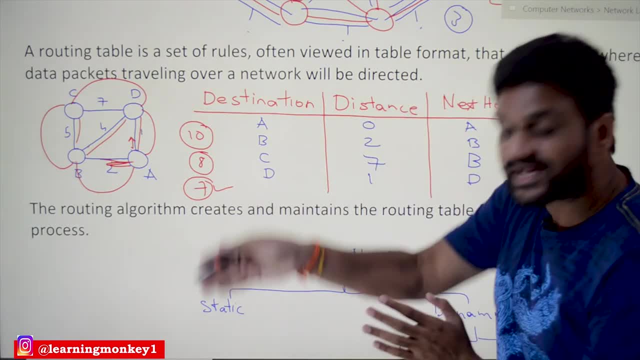 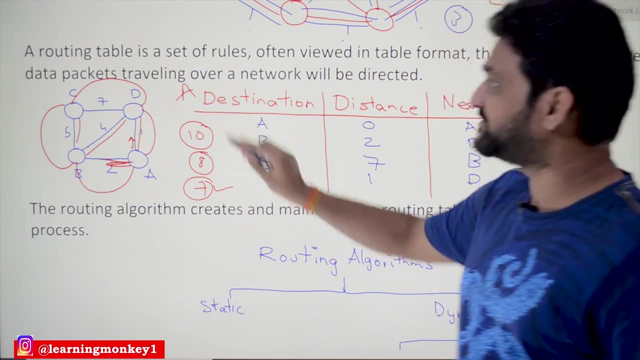 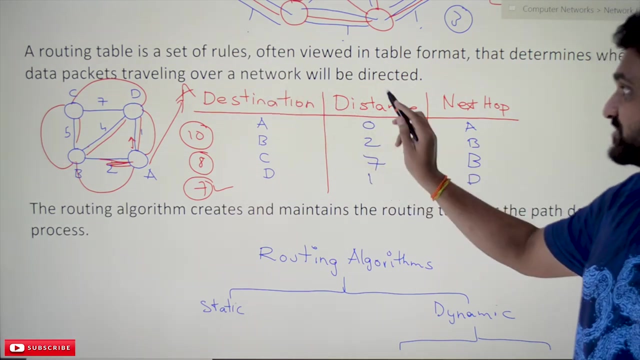 decision to for the data packet to get transmitted will be decided. okay, so let's try to understand that by using this table, and this table is there at the router, a okay, so what it consists of, the table consists of destination column, distance column and next hop column. so these are three. 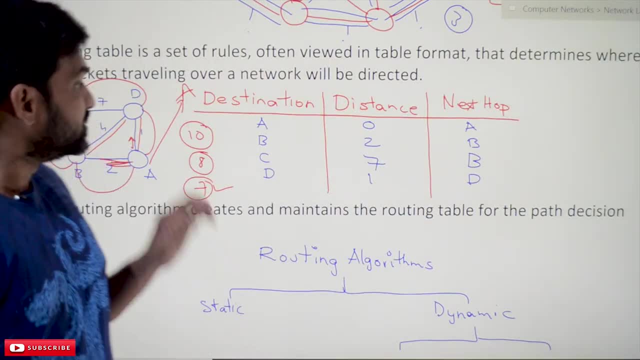 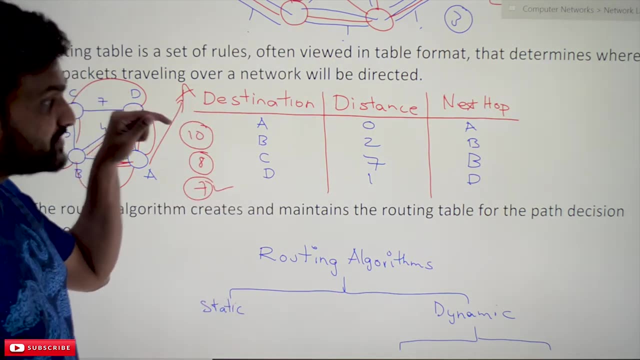 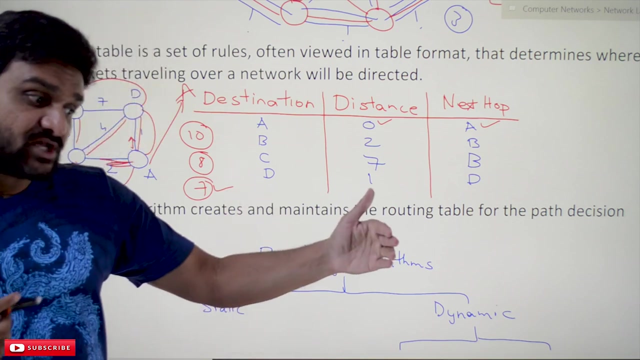 three columns that will be there in any routing table. so what the destination means. from A to A, in order the packet to get transmitted. from A to A, means it did itself. the distance is 0 and the next hop, next hop, means the router to which the packet has to be transmitted in order to transmit from A to A there. 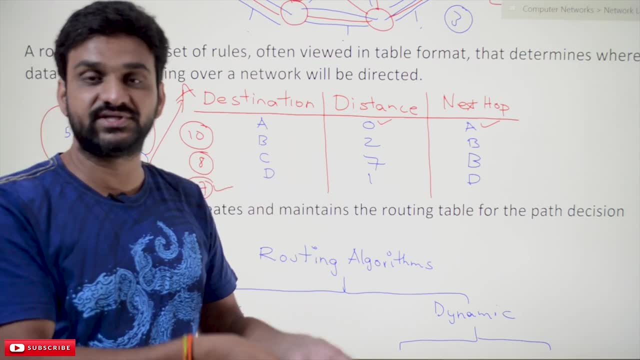 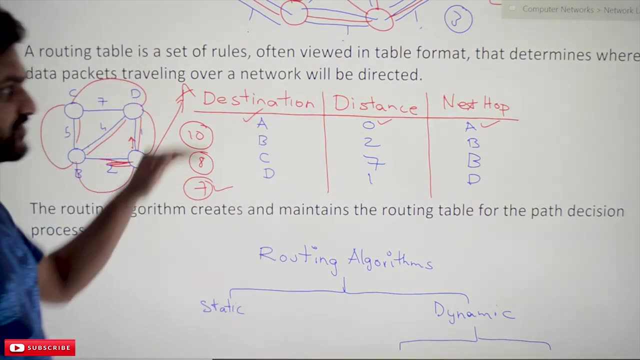 is no need for us to transmit to any other router. it has to be there on A itself. from A to A means here itself, so that is that will get maintained in one of the rooms, the next row, if you want to transmit the packet from A to B all. 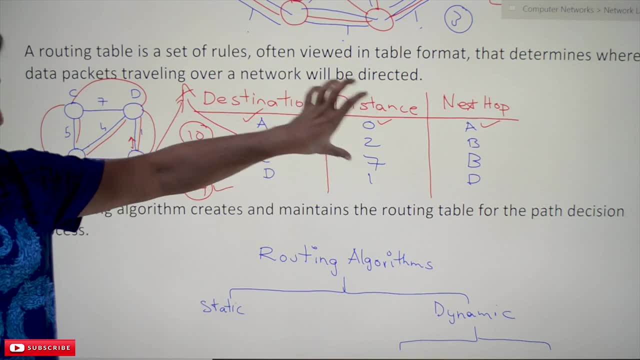 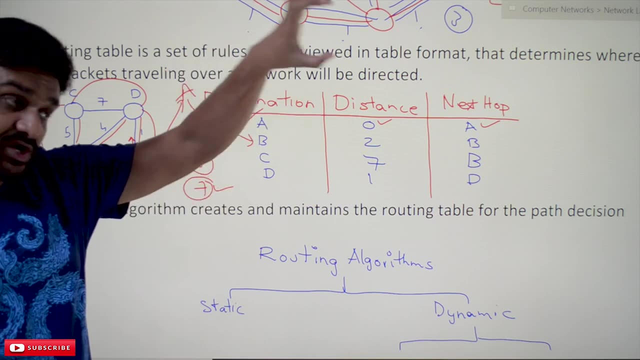 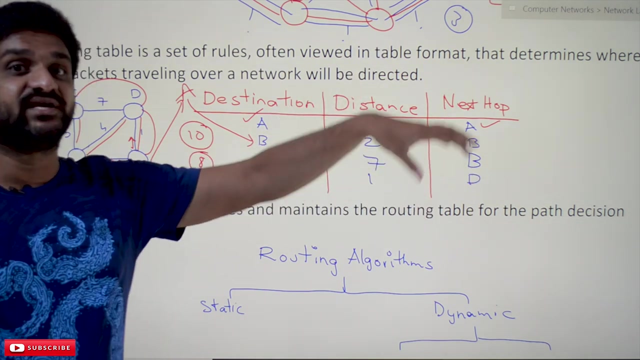 counters in the network. so the route distance vector- sorry, routing table- is going to have all the routers, the interconnection of all the routers, all the routers values will be there in the routing table. so that is the very important point to understand. for example, if this entire whole 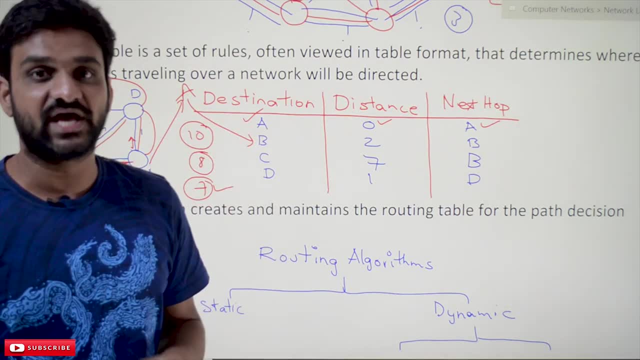 dish is a chain or if it is upö command, and then if you have 있고요 and all sort of so. for example, body of the 2019 standard in is getting connected by 100 routers means usually it will not happen in that way. So all the 100. 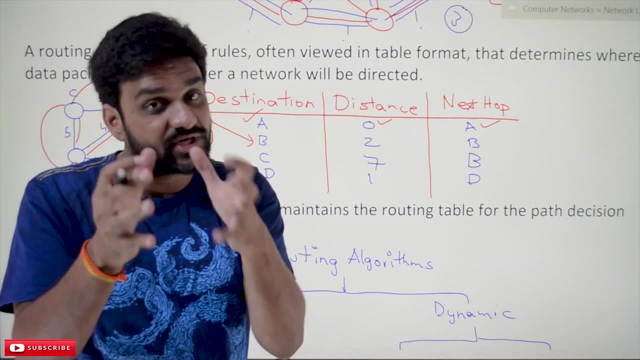 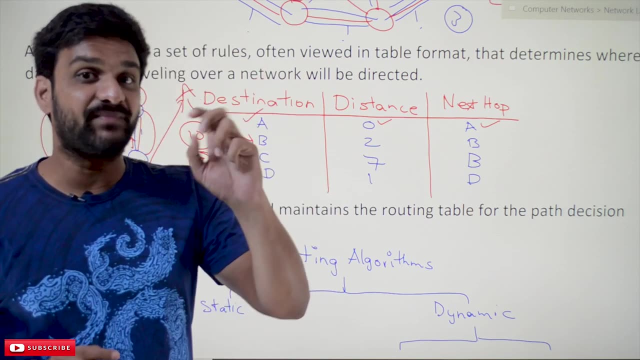 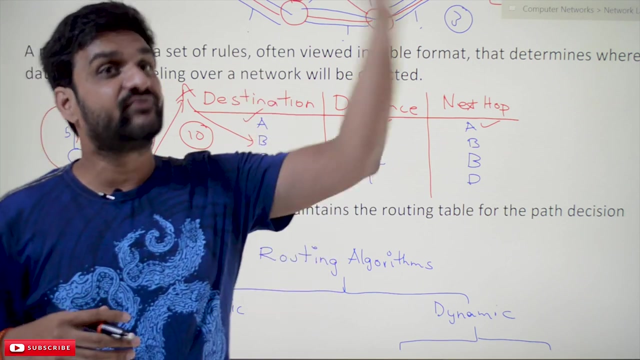 routers. details will be maintained at each and every router, So try to understand that point. each and every router, For example, if you are getting transmitted, the packet is getting transmitted away from India, So that router through which this entire world is getting 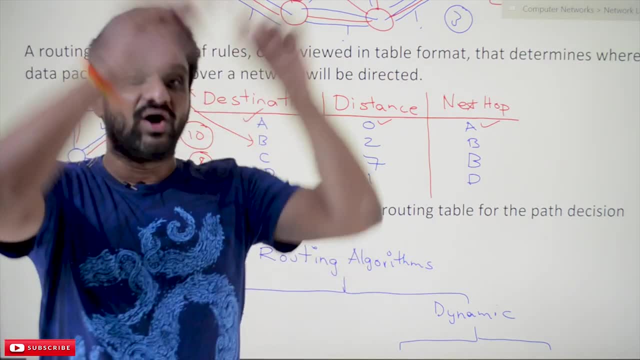 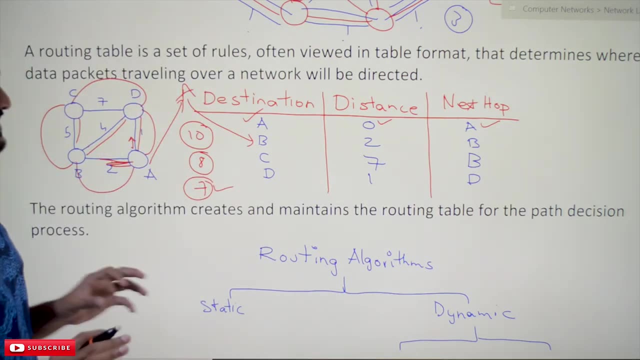 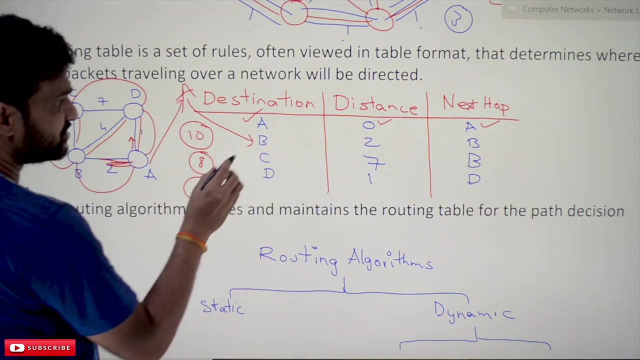 connected at that router. it will have the details of all the routers in this entire world. So based upon that it is going to decide. So do not go deeper at this point of time. it is not required So now, from A to B in order to transmit from A to B, what is the best path? is it this way? 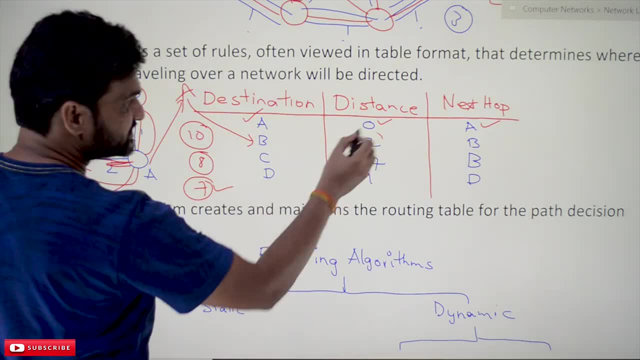 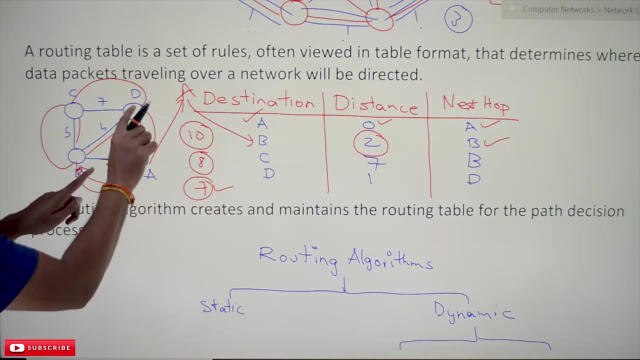 no, it is from directly to B, So the distance is 2 and the next hop is going to be B. Similarly, A to C. There are two possibilities, one to D and the other one is to B, but the best path is so, even though it. 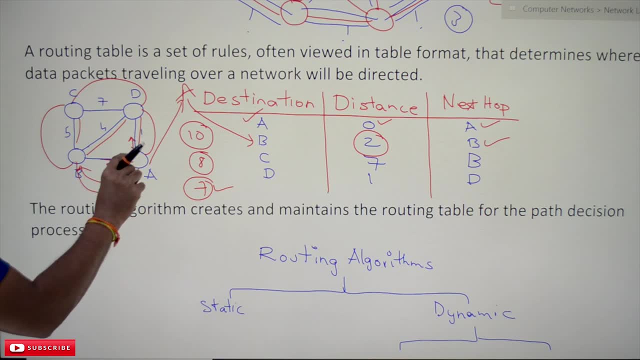 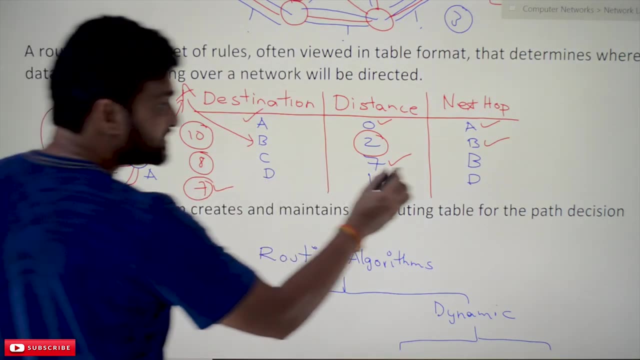 is one. it is going to take longest path, So we have to decide based upon the shortest path. So the distance is 7: 2 and 5: 7. the next hop is going to be D. Similarly, from D to A to D, in order to 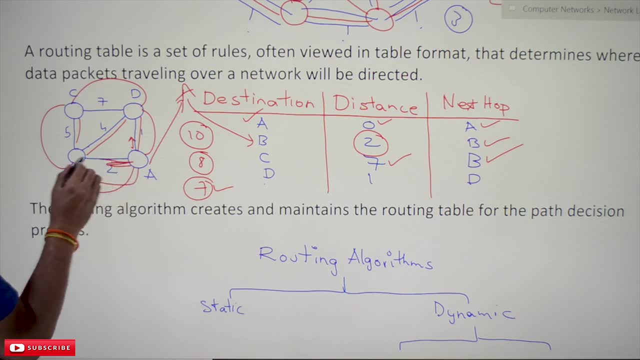 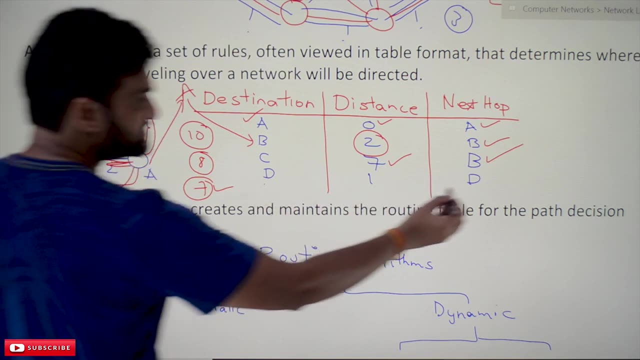 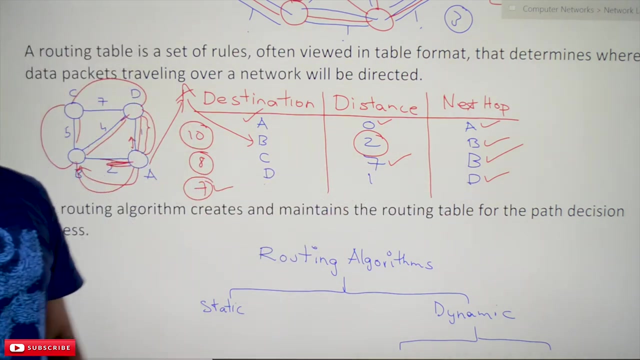 transmit from A to D. the best path is: we can go either this way or this way, or this way, this way, this way, But the best way is, the best path is this one. So it is a D in order to transmit from A to D. the next hop is going to be D and the distance is 1.. So this is what we call it. 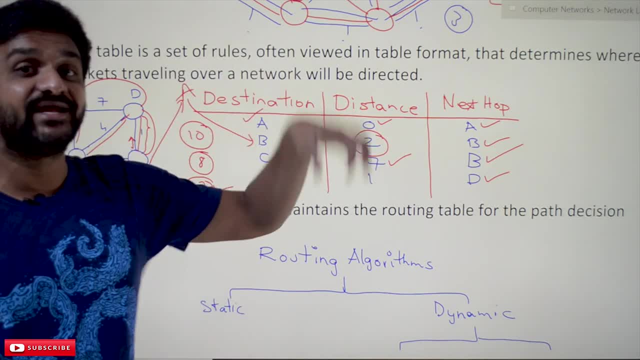 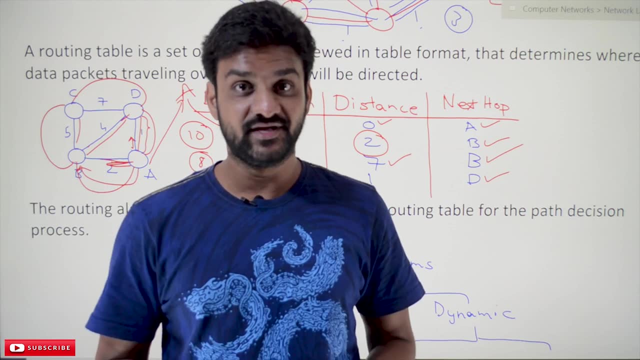 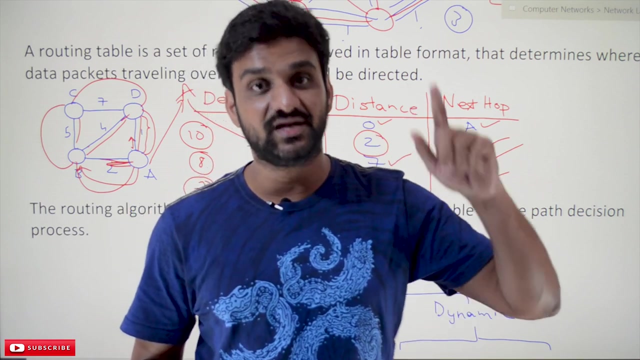 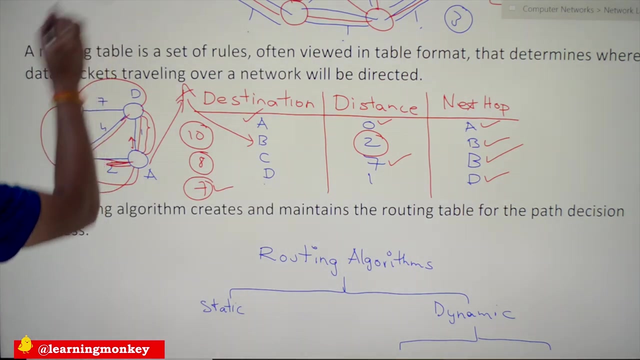 as a routing table and this table will get maintained in each and every router. So how the routing table is getting generated. it is our next question: How the table is getting generated by using routing algorithms. it is generated by using routing algorithm. so what is meant by routing algorithms? see here: routing algorithm creates and. 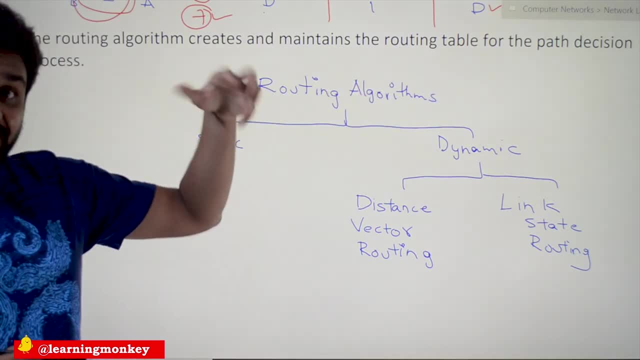 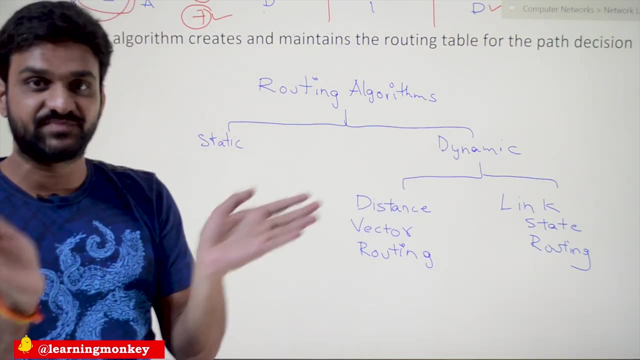 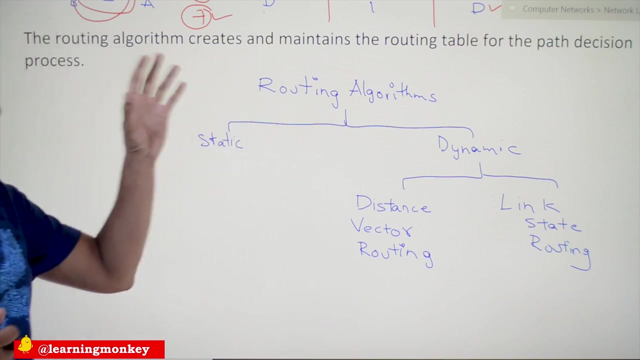 maintains the routing table. routing algorithms creates and maintains the routing table. for why? what is meant by maintenance? for example, if one of the line has been disconnected, so again the routing table will get regenerated. so that is what we call it as maintenance, so those routing tables can be routing. 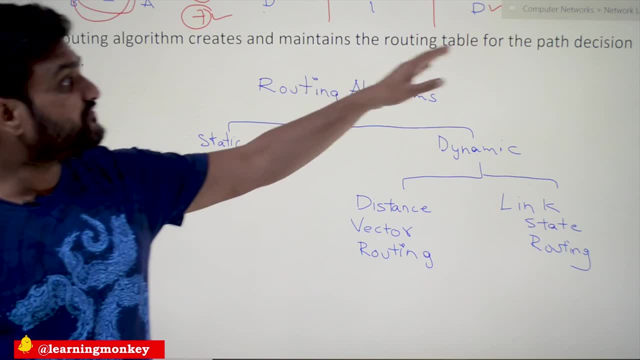 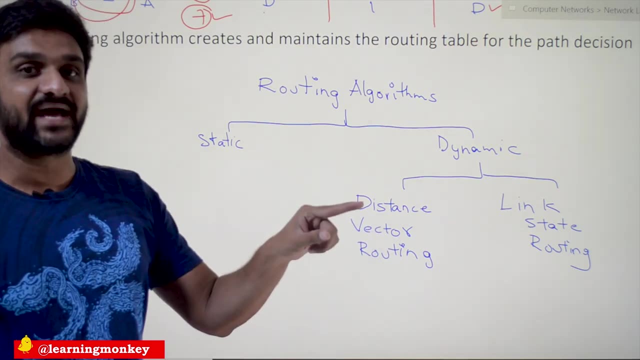 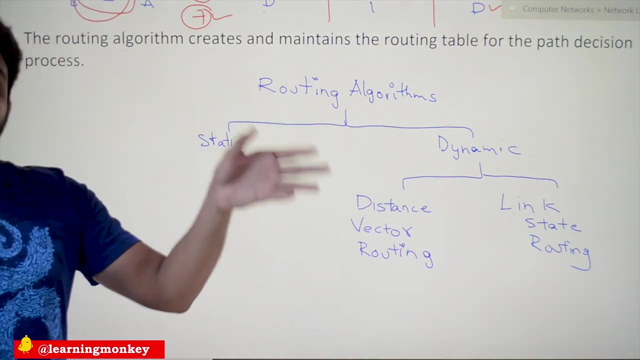 algorithms are going to create and maintain routing tables for the path decision process, for the path decision process, in order for the packet to transmit to the next router, so that path decision-making process is decided by the routing table and routing table and that routing table is generated by the. 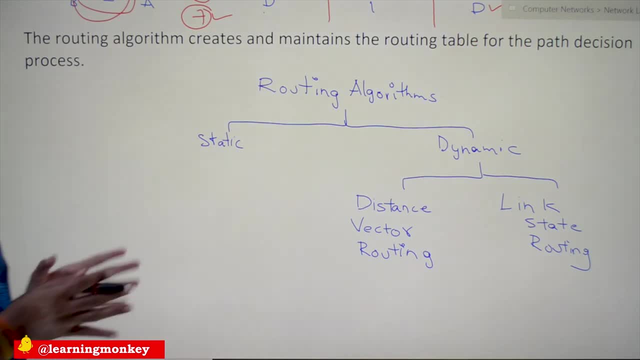 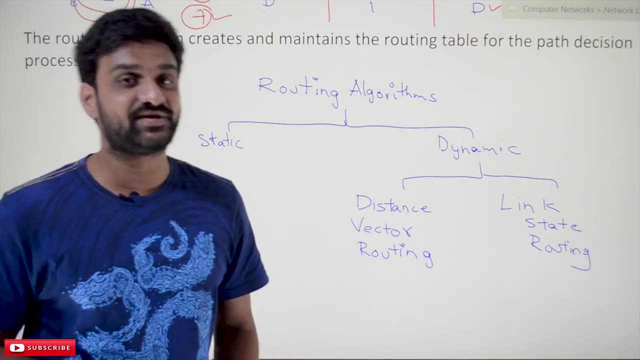 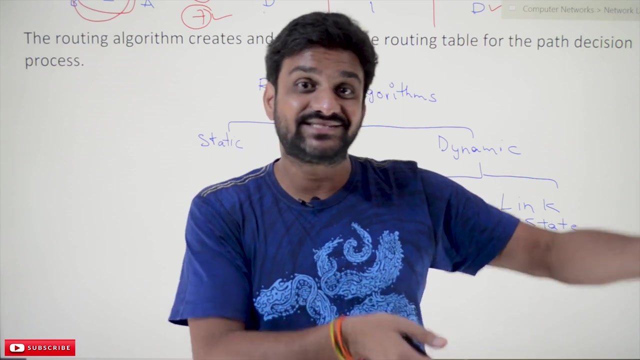 generated by the routing algorithms. there are two ways in which these routing way tables can be generated. one is static and the other one is dynamic. so what is this static means? so the network administrator will go to each and every router and they will pay. they will place that routing algorithm, now the routing table. so is it?